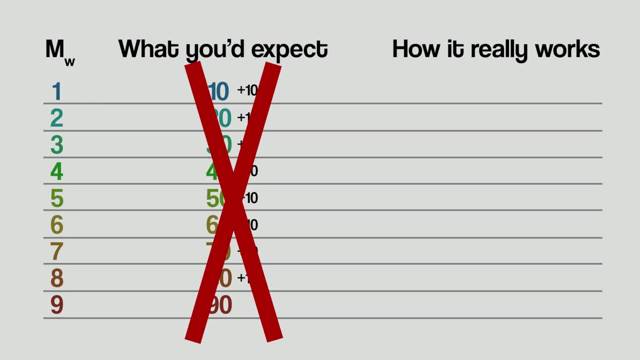 numbers again, just like before. our magnitude 1 earthquake releases 10 units of energy. To get to the next magnitude, we don't add 10, we multiply by 10.. That means a magnitude 2 would release 100 units of energy. 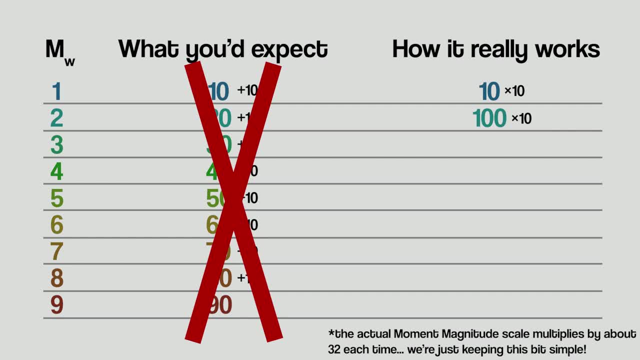 From there we multiply the number by 10 again, So magnitude 3 would be 1000 units of energy. Then we multiply 1000 by 10, so a magnitude 4 would release 10,000 units of energy. Woah, woah, hold up a second. we're only at magnitude 4 and already the earthquake. 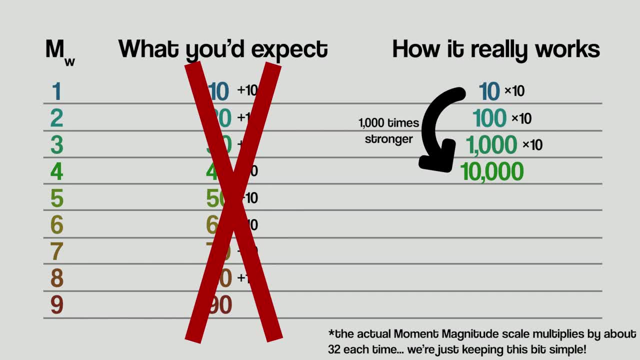 is 1000 times more powerful than magnitude 1.. Well, let's keep this going. Magnitude 5 would release 100,000 units of energy. Magnitude 6, 1,000,000.. Magnitude 7, 10,000,000. 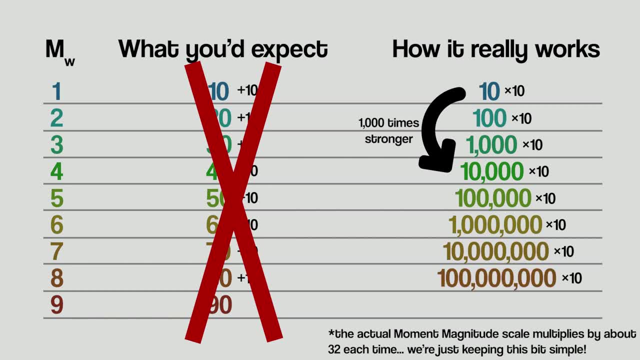 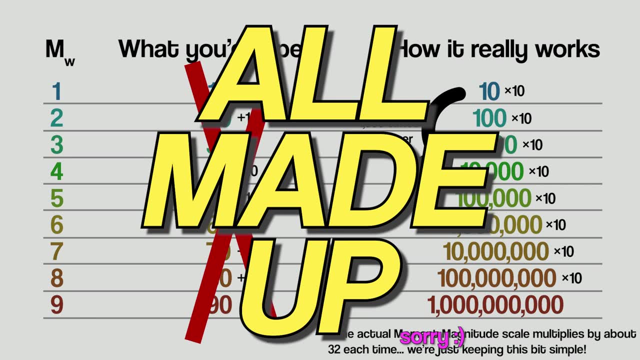 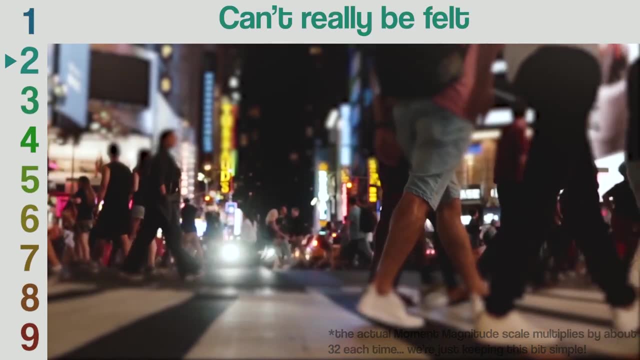 Magnitude 8, 100,000,000. And magnitude 9 would release 1,000,000,000 units of energy. But those are all made up numbers. How strong are real earthquakes on the moment? magnitude scale- Well, magnitude 1 and 2 earthquakes generally can't even be felt by people. 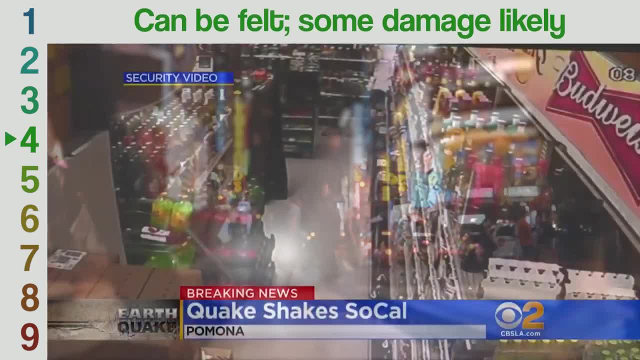 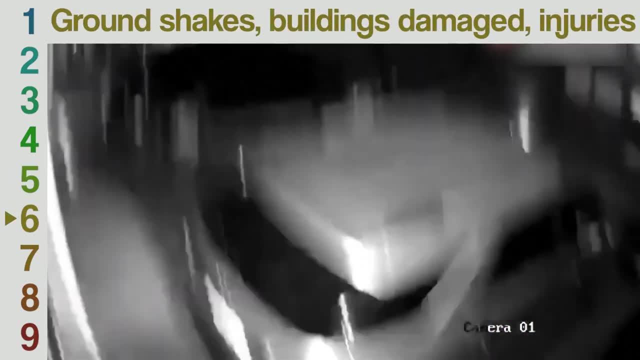 And the same goes for magnitude 3. some of the time, A magnitude 4 earthquake is where you'd normally feel it, and a 5 is where you'd expect to see some damage. Magnitude 6 is what you'd call a medium strength earthquake. 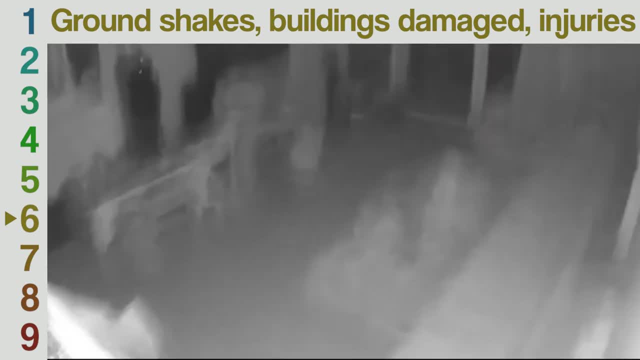 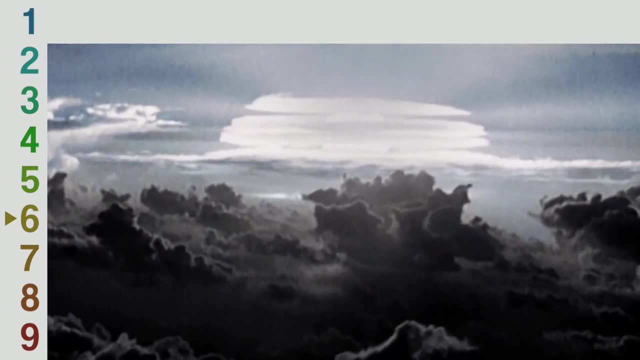 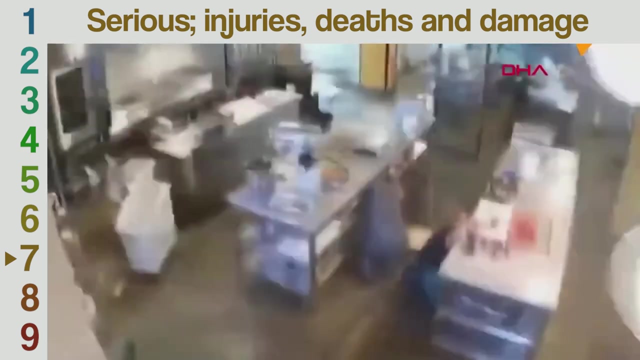 The ground would definitely shake and you'd expect quite a lot of damage to be caused. The nuclear bomb dropped on Hiroshima released about the same amount of energy as a magnitude 6.5. And we're still not done. Magnitude 7 earthquakes are where things get really serious. 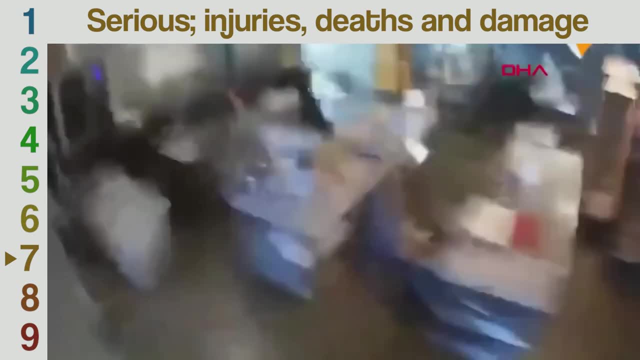 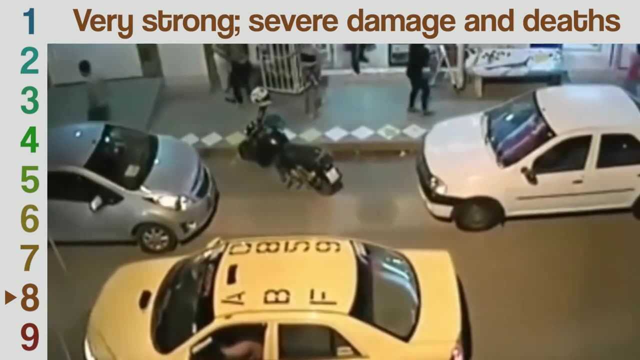 Happening on average about once per month, They are often strong enough to cause a lot of injuries, deaths and damage. Magnitude 8s are significantly stronger than the already powerful magnitude 7.. Happening only once per year on average, these earthquakes will cause an enormous amount. 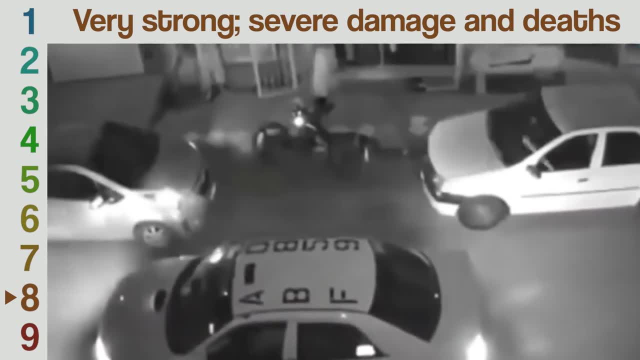 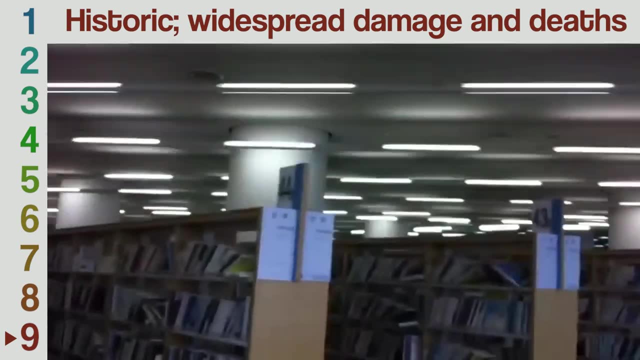 of damage to structures, as well as significant injury and loss of life in most cases. And then we get to magnitude 9.. These earthquakes are extremely rare, Happening roughly 1 to 3 times every 100 years, And, as you can imagine, they are devastating.